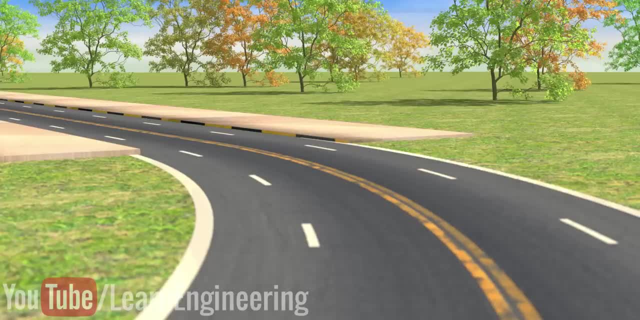 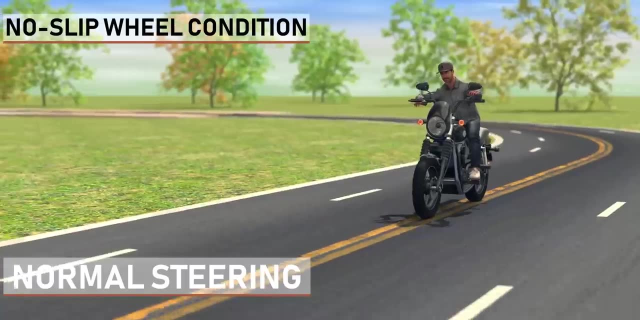 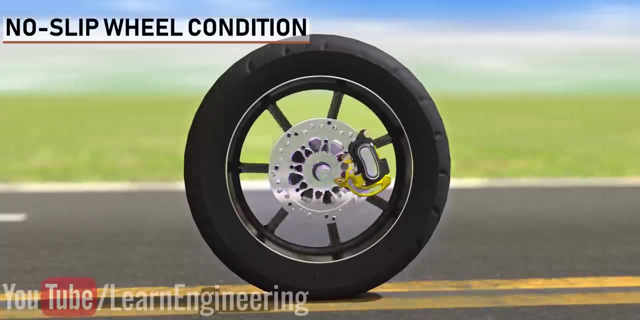 Let's explore. Before understanding the physics behind counter-steering, we need to understand the physics behind normal motorcycle steering and no-slip wheel condition. First, let's explore what is meant by this no-slip condition. The wheels are always trying to attain a non-slip condition, which means that the wheels should have no relative motion with 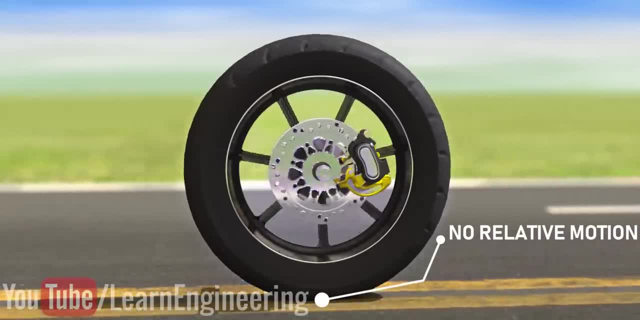 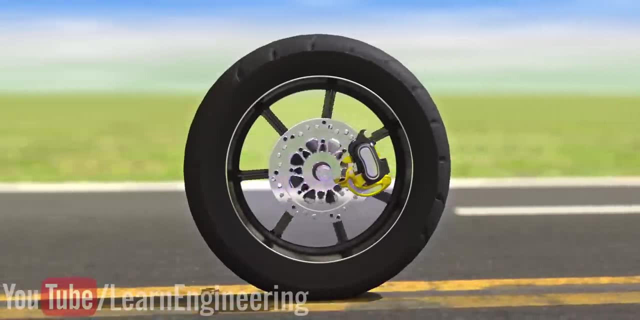 the road. Since the road is at rest, the wheel contact point should have zero velocity. But how is zero velocity possible for a moving wheel? It is possible because the wheel has two kinds of motion: A translational motion, where the wheel is at rest, and a non-slip motion, where 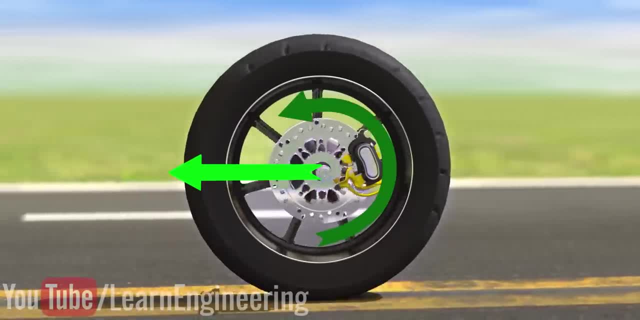 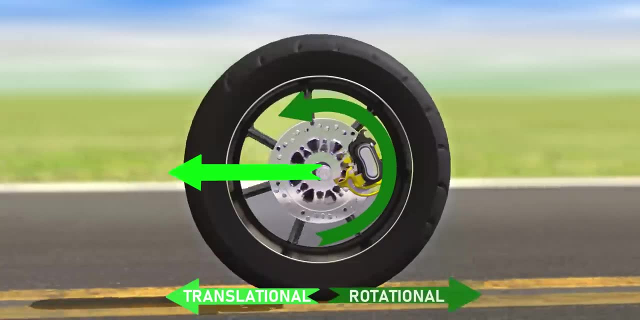 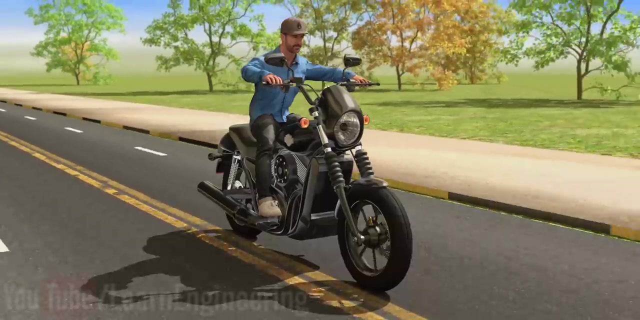 the wheel is at motion along with the vehicle and a rotational motion on its own axis. You can see that it is possible to make the resulting velocity zero at the contact point, since the translational and rotational velocities are in opposite directions. In normal steering, to make a right turn, what we do is just turn the handlebars towards the right. 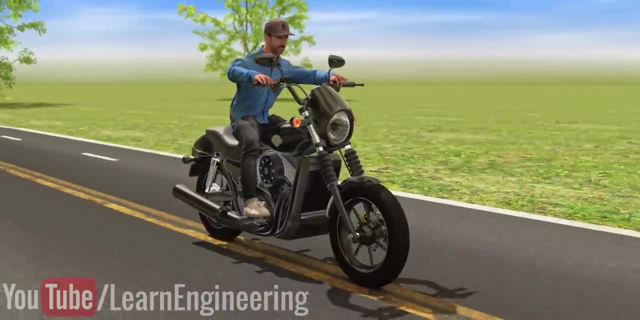 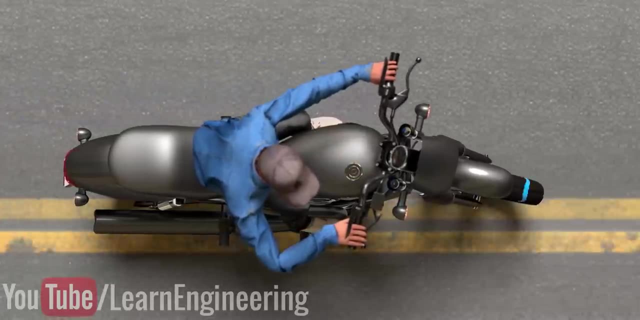 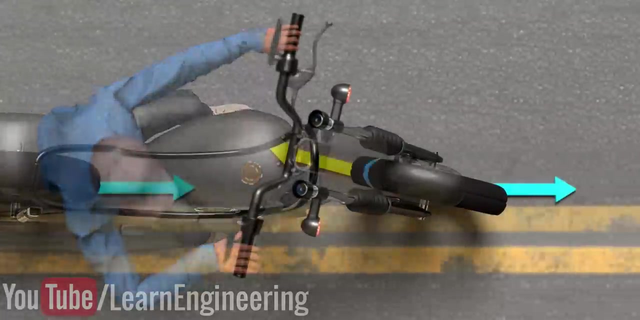 and lean the motorcycle inwards. Let's analyze the normal steering operation in a step-by-step manner to understand the physics behind it. Assume that even after turning the handlebars, the vehicle moves straight ahead. Here, if you check the front wheel, it will not meet the no-slip condition. 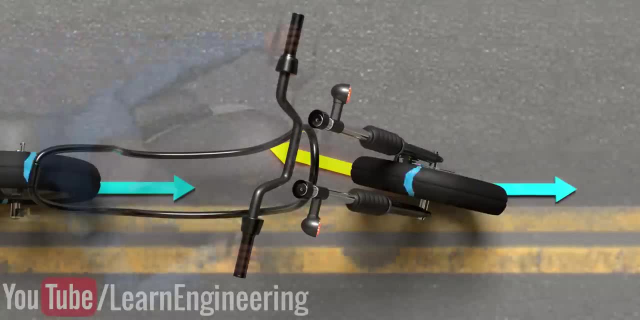 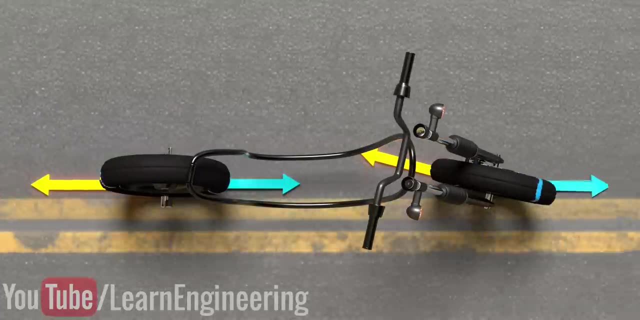 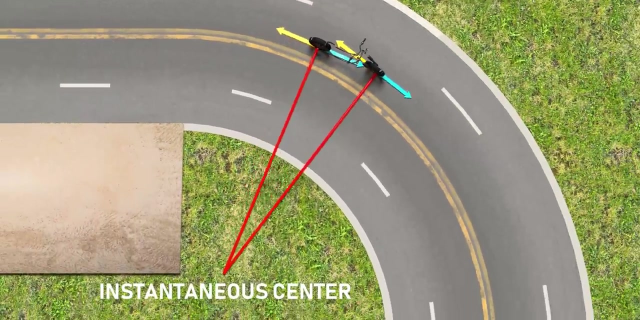 since the wheel and vehicle velocities do not cancel each other out, The only way to solve this problem is by making the translational velocity inclined as well. This is possible when the whole motorcycle makes a turn around an instantaneous center. How to solve the problem? 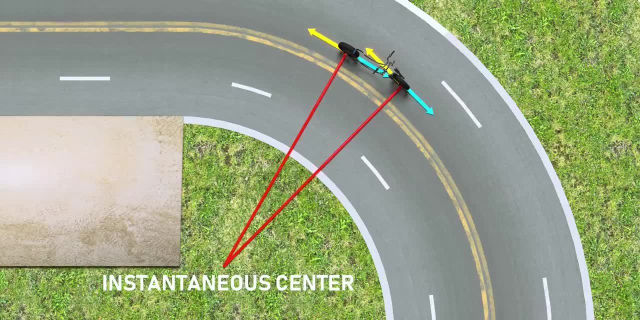 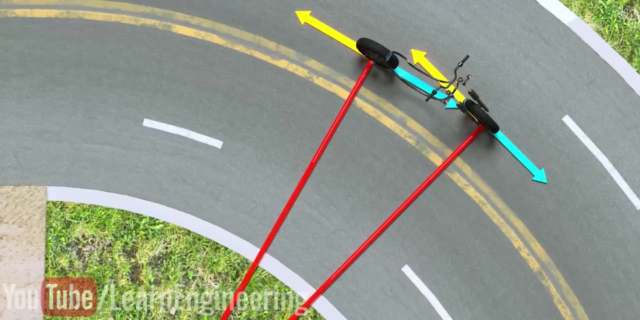 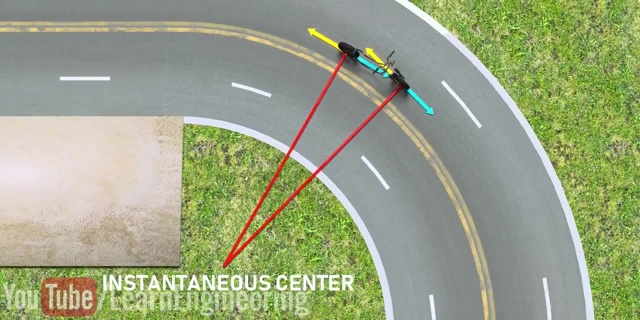 The instantaneous center should be at the intersection of both the wheels' normal lines. It is clear that when the motorcycle makes a turn in this manner, both the wheels easily satisfy the no-slip condition. In short, the no-slip condition forces the motorcycle to make a turn. 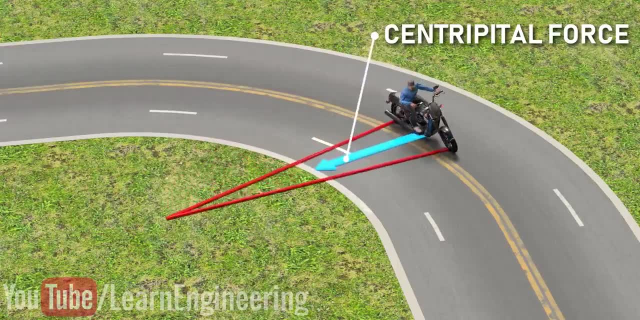 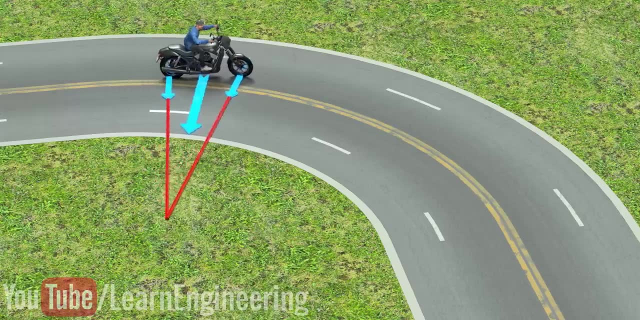 However, a centripetal force is needed for any object to make a turn. This centripetal force is provided by the frictional force between the tire and the road. Let's do the torque balance. Let's do the torque balance of the motorcycle at one point during the turn. 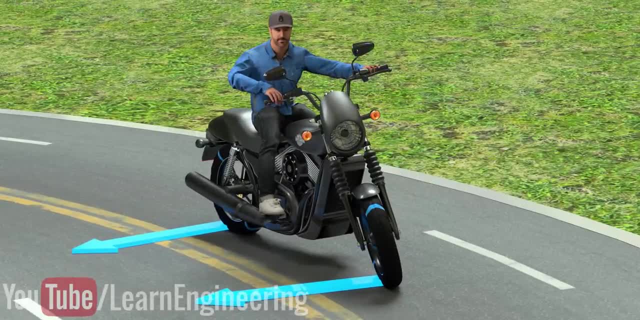 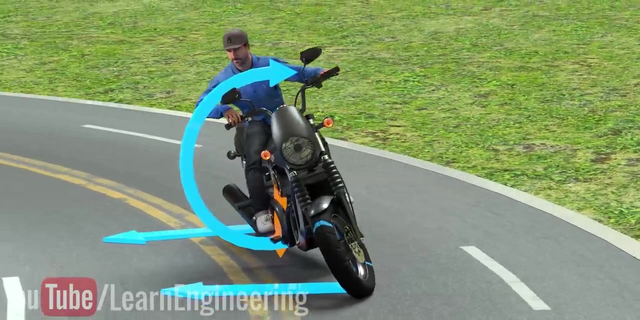 You can see that the vehicle is not stable in this position. The torque produced by the frictional forces will turn the motorcycle down. The only way to balance this torque is by leaning your motorcycle inwards. You can see how the gravitational and normal forces act in the inclined motorcycle position. 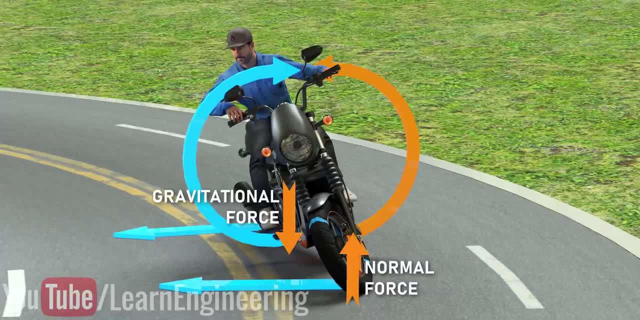 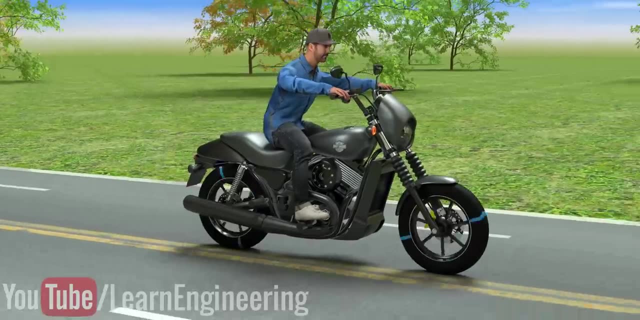 This will produce another torque which can counter the torque formed by the centripetal force. This is the way you normally turn the vehicle. You turn the handlebars to balance the torque produced by the centripetal force. just lean the motorcycle. 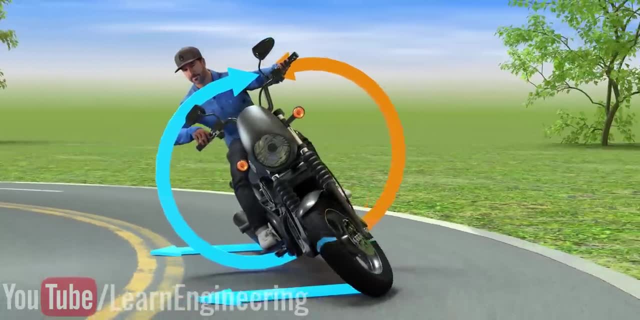 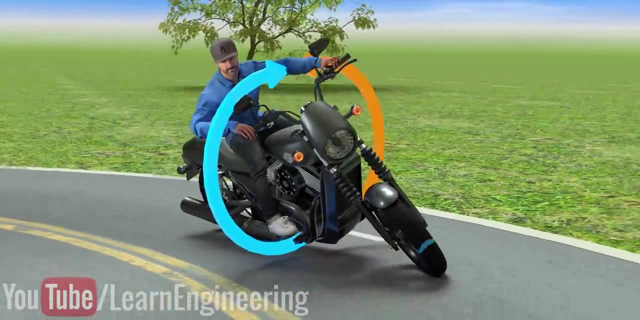 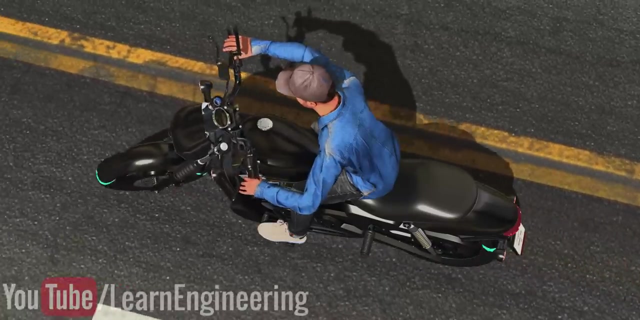 Here the rider has to adjust his body position to achieve the lean of the motorcycle. Note that the handlebars turning and the leaning operation happen simultaneously and are in perfect balance. How is counter-steering different from normal steering? In counter-steering, you turn the handlebars. 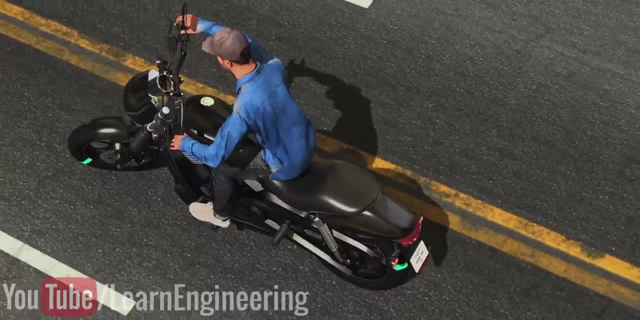 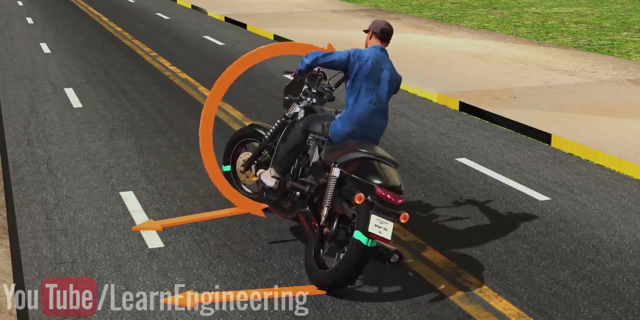 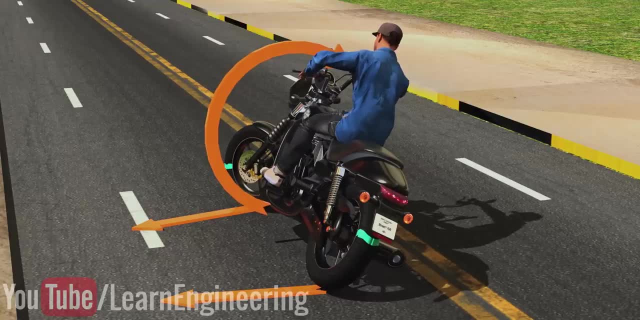 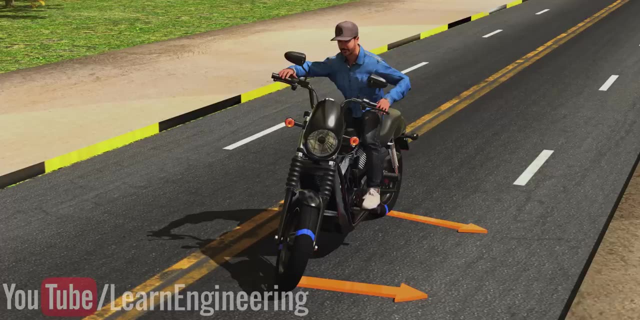 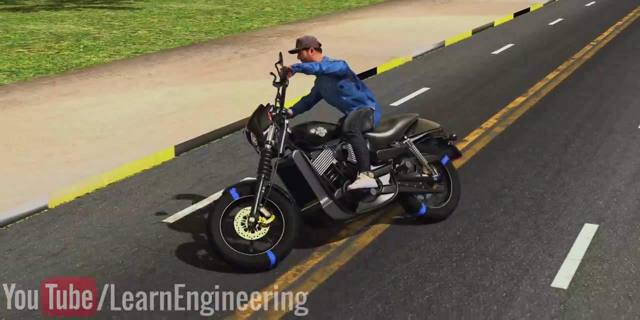 In short, the motorcycle achieves a lean in the opposite direction for a moment. This lean is sufficient to achieve a perfect turn in the opposite direction. One thing to be noted here is that during the lean operation, the driver cleverly adjusts the angle of the handlebars so that it is suitable for a perfect 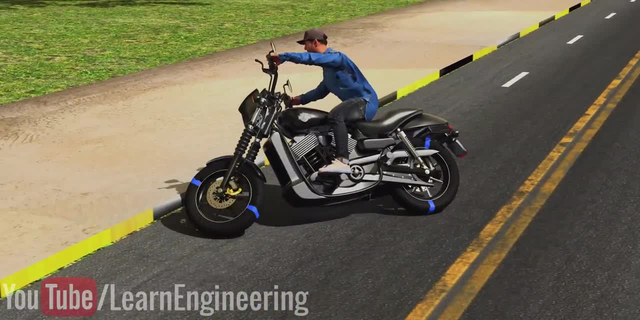 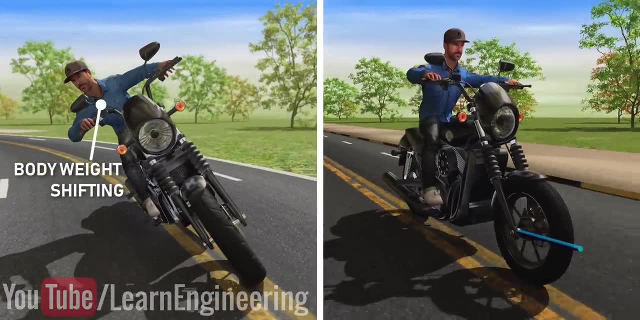 no-slip condition. In short, in normal steering, the lean of the motorcycle is achieved by shifting your body weight. In counter-steering, the lean is achieved by the motorcycle's instability caused by the centripetal force. In counter-steering, the lean is achieved by the motorcycle's instability caused by the centripetal force. 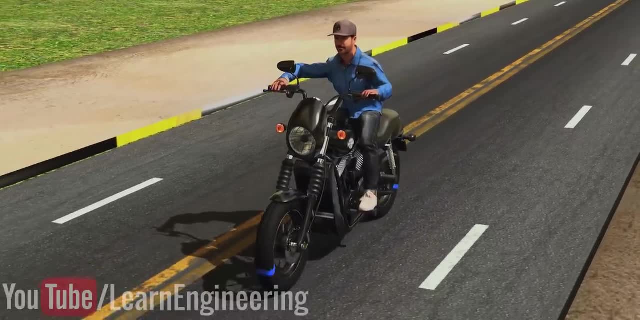 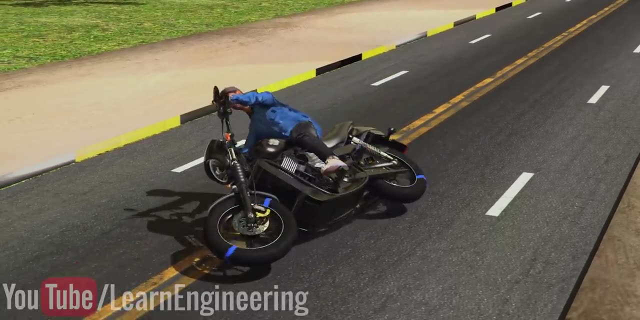 Obviously, counter-steering is a quicker operation but slightly risky. If you don't steer the handlebars back to the proper angle during the leaning operation, you are going to fall down. This is why proper practice is needed to master this instability. 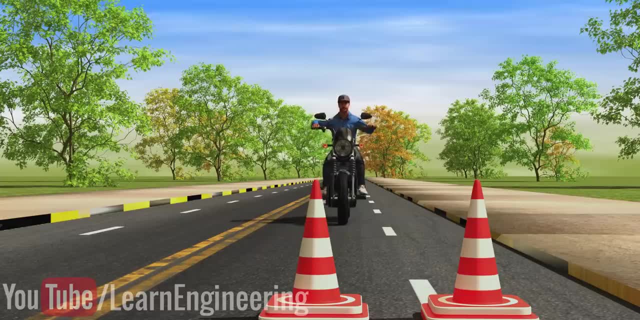 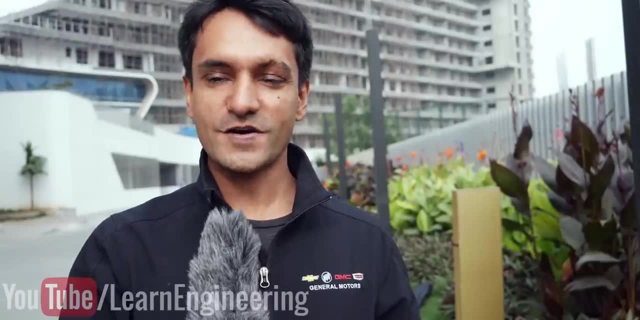 Counter-steering is quite handy to avoid sudden obstacles in the road. Counter-steering is quite handy to avoid sudden obstacles in the road. Let's see how it works in practice. The trick of counter-steering is that you turn the handle but don't lean.